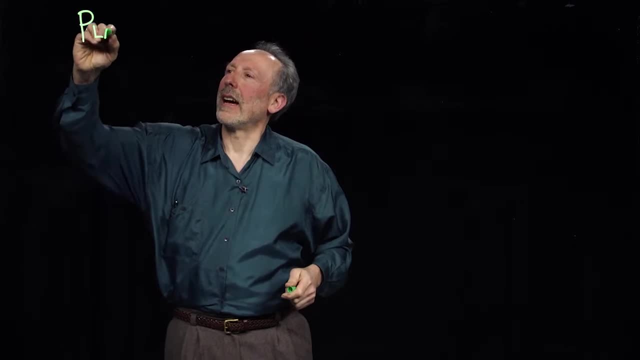 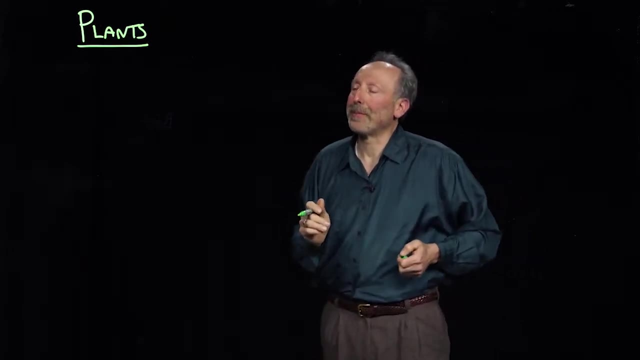 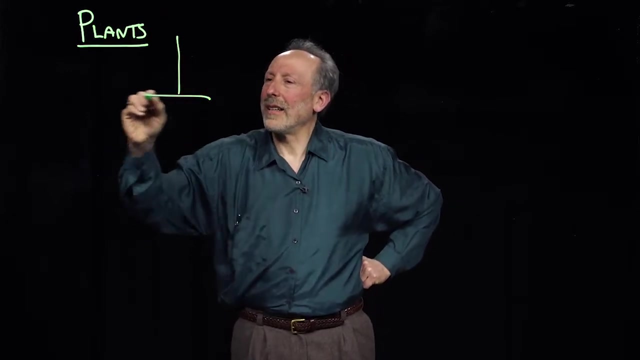 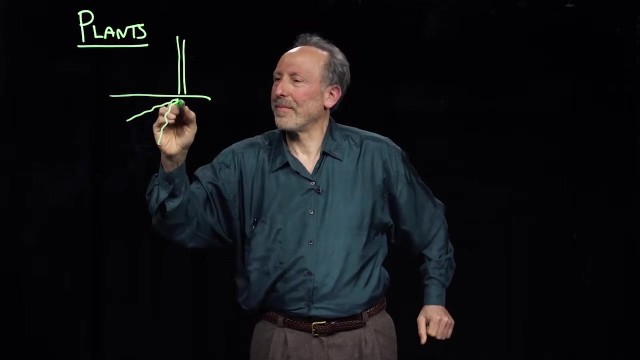 like to talk a little bit today is about plants and how plants are a fundamental piece of when we talk about the soils and unsaturated zone, And so really starting with when we have our plant and our soil, this is obviously a highly refined diagram. what we're going to have are these roots And the thing about roots. 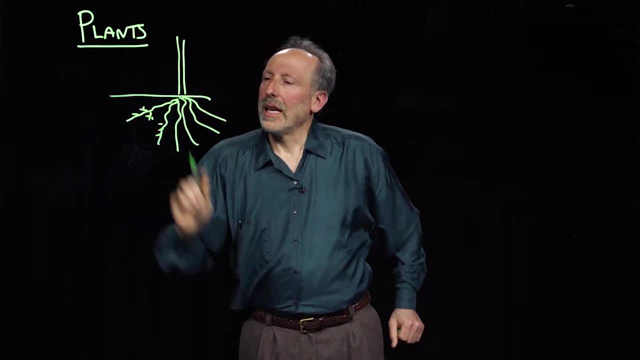 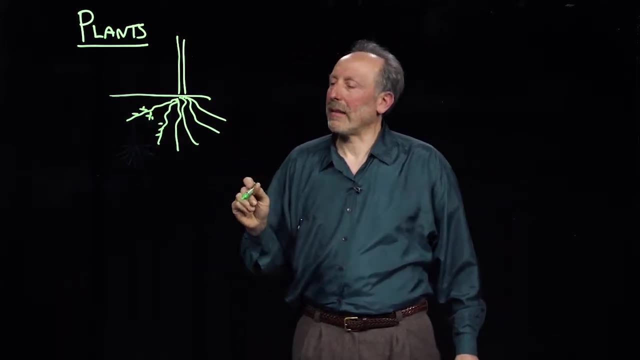 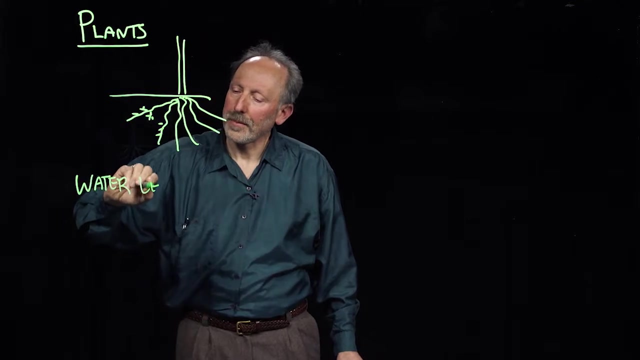 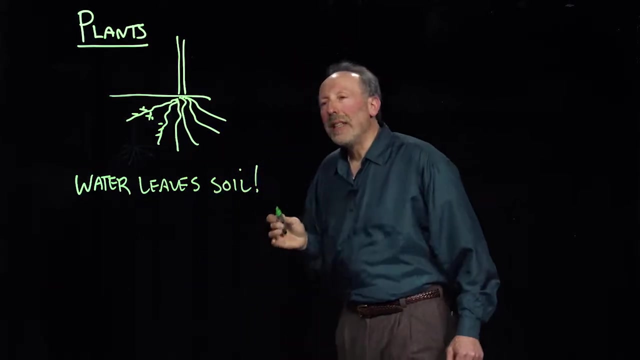 is they have fine structure coming off of them. Roots have a tremendous impact on many aspects of water movement in soil. Most dramatically, roots are going to impact the way water and water leave soil. So the deal is that, while we can have infiltration processes where water, percolates, due to gravity and capillarity, etc. the wetting fronts typically occur under very near saturated conditions, So there's a lot of water. it can flow. When the water is leaving the soil, the soil is actually rather dry typically. 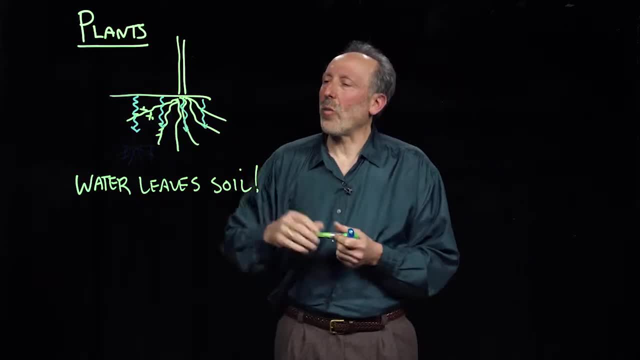 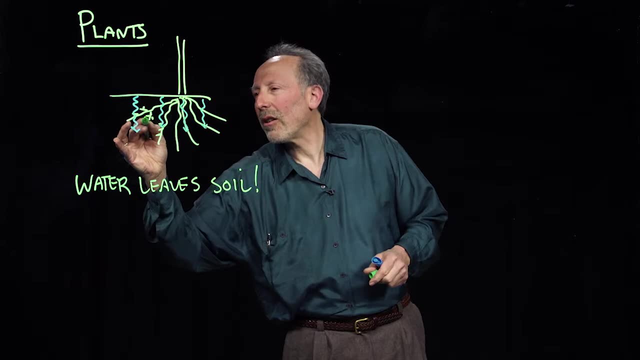 It's dried out where it feels firm, And so the only way for water to get out of that soil is for the roots essentially to chase the water, And so, in fact, the length scale of water moving to the roots is on the order of 100 times. 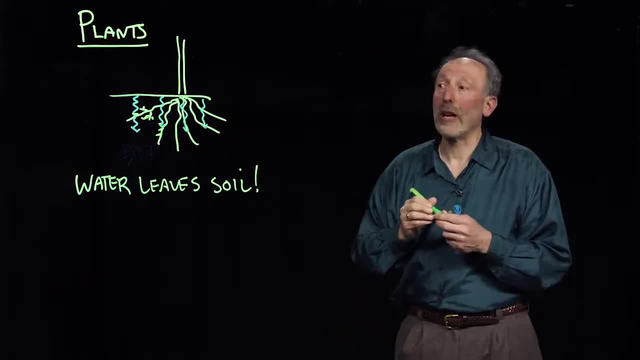 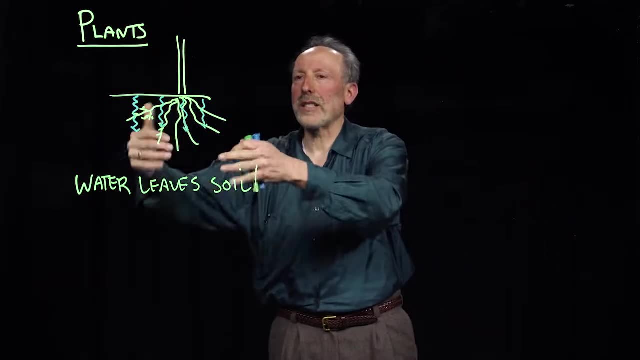 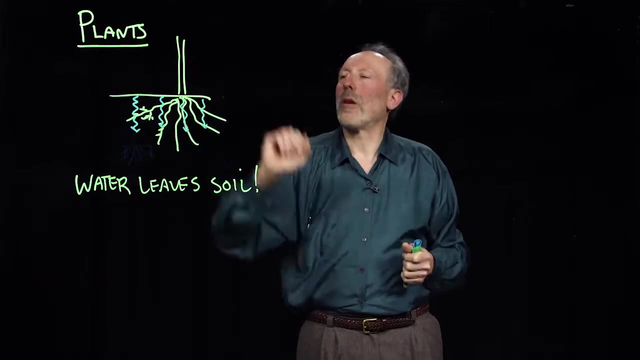 shorter than the length that water came to the roots. So the water leaving through the roots means the roots have to be distributed through the entire soil profile, whereas the infiltration process happened without respect to the plants. So we immediately see that the departure of water from the soil is not just, as if it was. 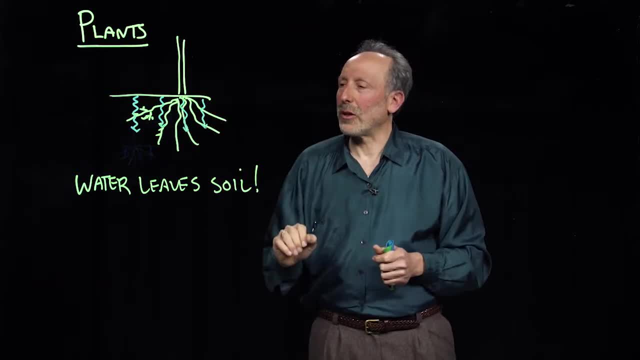 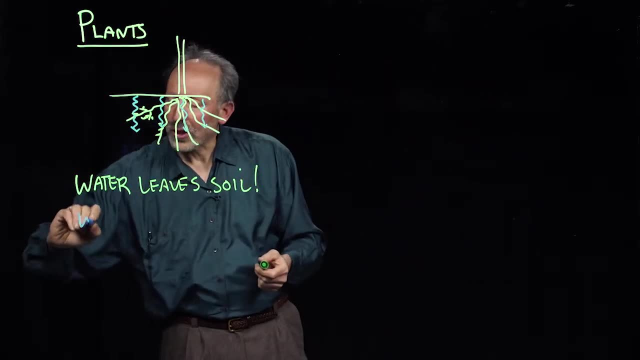 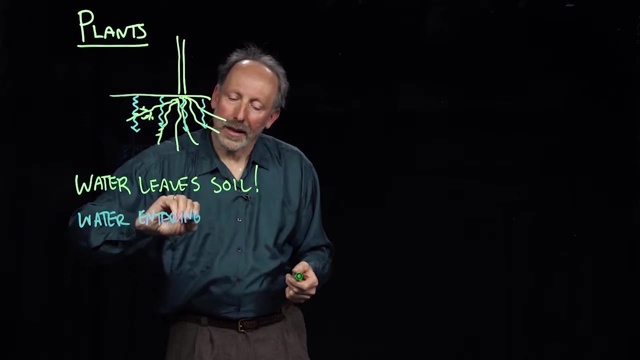 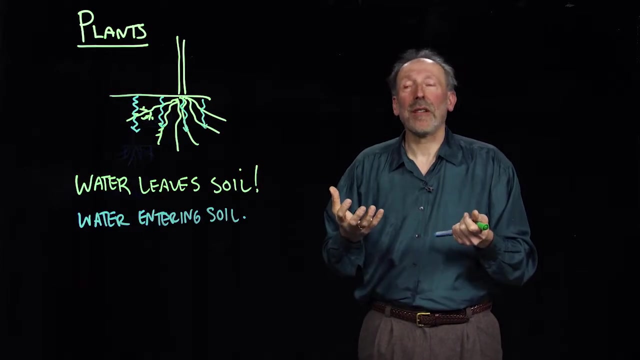 a flat surface with no biota on it. The plants are absolutely critical. So the way water leaving the soil, But it also does impact the way water enters the soil. How is that? Well, Okay. So if we took a silt, or like a flower, textured of material and packed it together and we 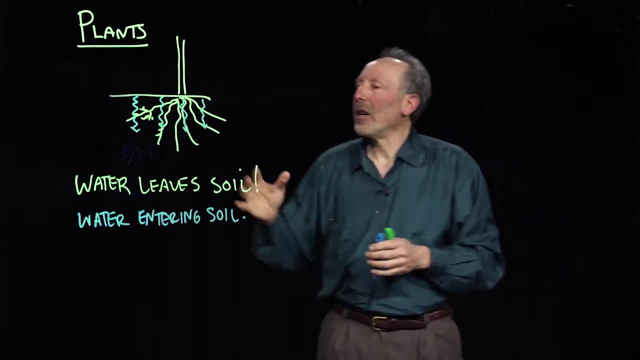 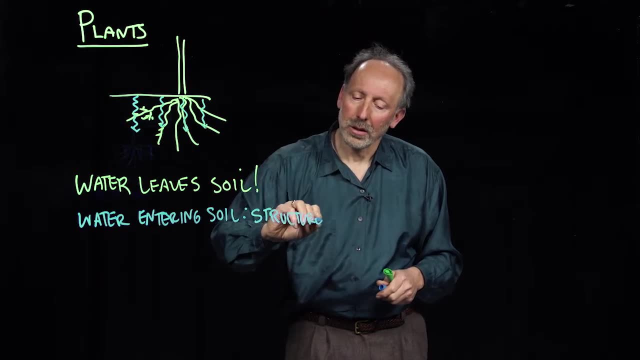 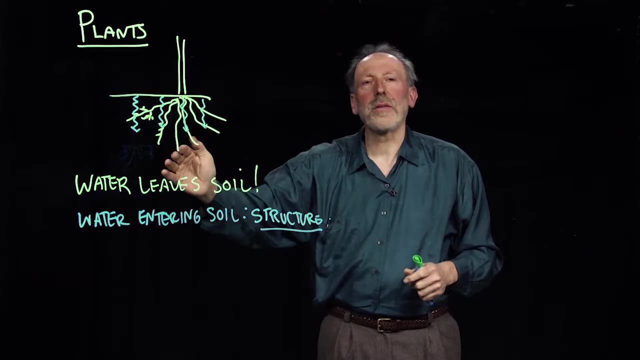 tried to pour water on it. water doesn't go in very well, And so, in fact, the key thing of water entering the soil often has to do with structure, And so structure means the way that clods of soil are organized, But structure is also provided by roots, and roots emanate from the surface, and they go.